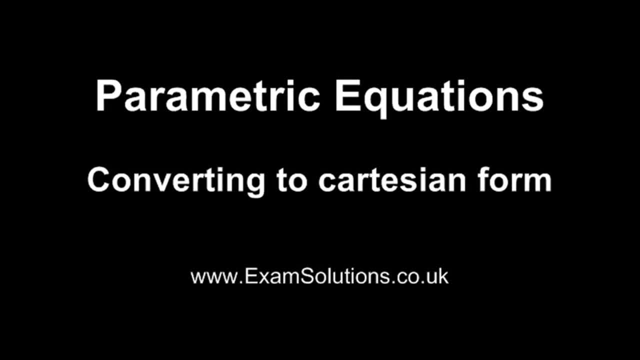 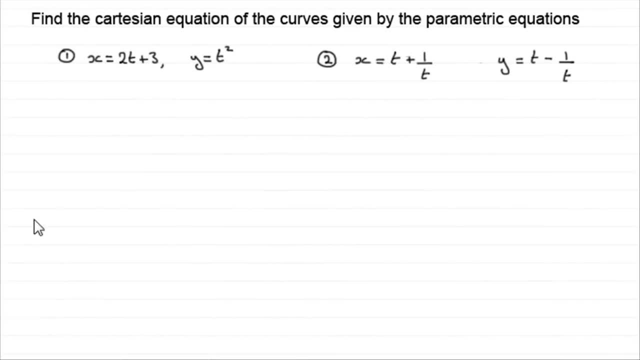 Hi, in this video, what I want to do is show you how we can convert a parametric equation into a Cartesian equation. I've got two examples here. The second example is a lot harder, though, to do than the first one. Now, when we're trying to get the Cartesian equation, what? 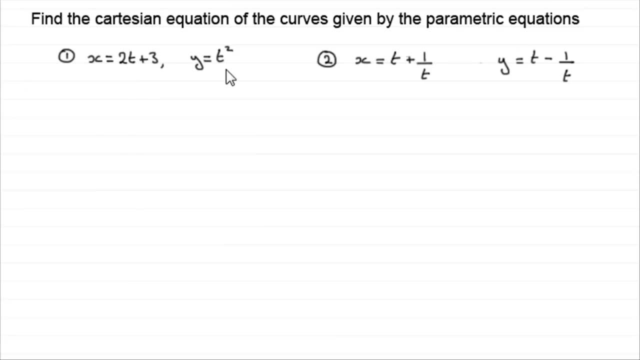 we've got to do is eliminate the parameter. In this case, the parameter is t. between the two equations We're looking to get an equation involving just y and x- And to do this in the first one. this is a fairly basic one. just to get started, What I would do is I'd 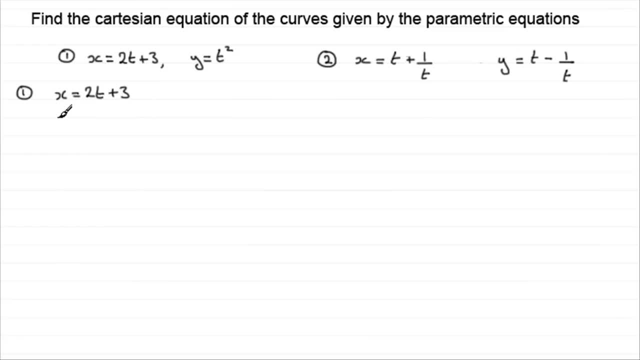 write the two equations out Again. we've got x equals 2t plus 3, and we've got y equals t squared, And I would number them 1 and 2 just for reference. Now what we need to do is take the easier of these. 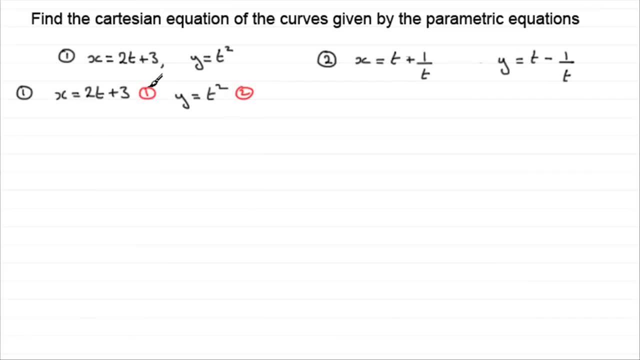 two equations and it has to be number 1 to make t the subject. It's a linear equation rather than the quadratic equation here. So I would say to the reader which equation I'm looking at, And in this case it's. 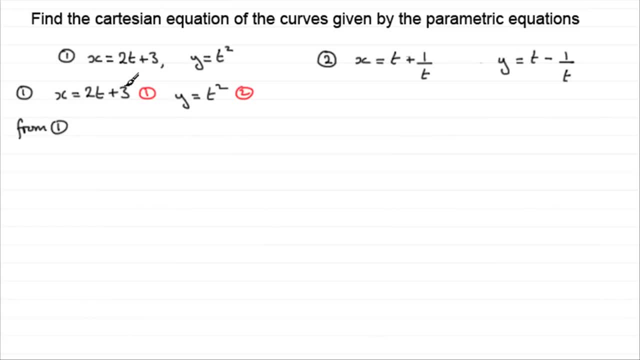 Subtract x from 1. And I'd make t the subject. I'd do that by subtracting 3 from both sides and dividing by 2. And that would mean that t equals x minus 3 all divided by 2. And with: 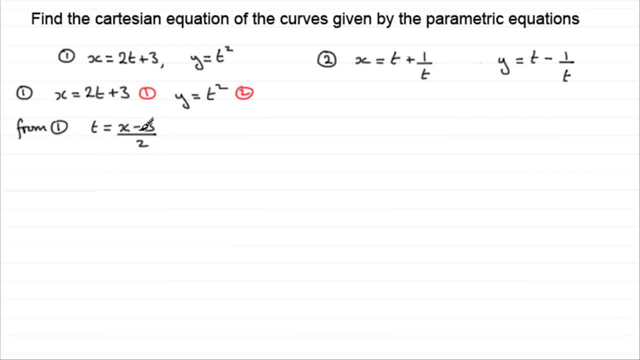 this equation, I can substitute t in terms of x into 2.. So, again, I would say that I'd just say sub into 2.. And what would I get? Well, we'd have x minus 3 divided by 2.. And 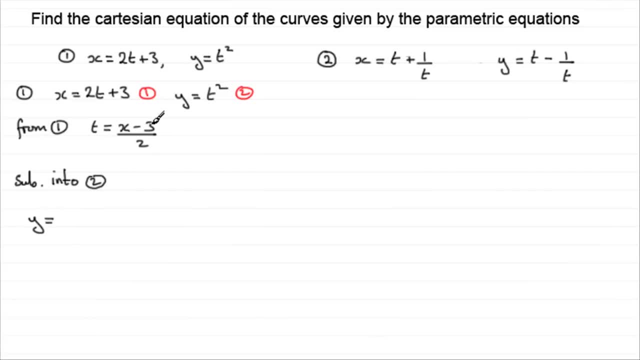 what would I get? Well, we'd have y equals t squared, which is going to be x minus 3, all squared over 2 squared. So we have x minus 3, all squared over 2 squared, which we might as well write as 4.. And I'd leave it like that. That's fine for our Cartesian equation. 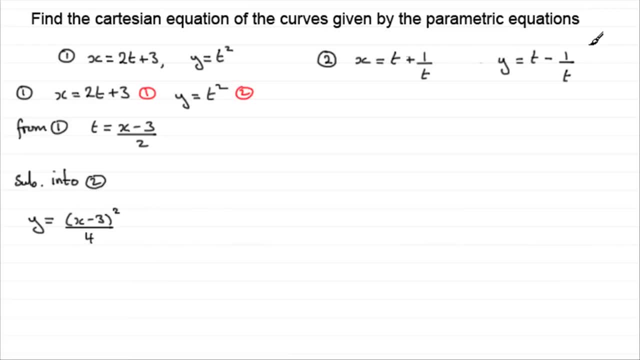 Now, when it comes to the second one here, as I said earlier, it is a lot harder to do. You might like to have a go, though, okay, but what I'm going to do is just write these equations out here and number them one and two again. Now, how are we going to? 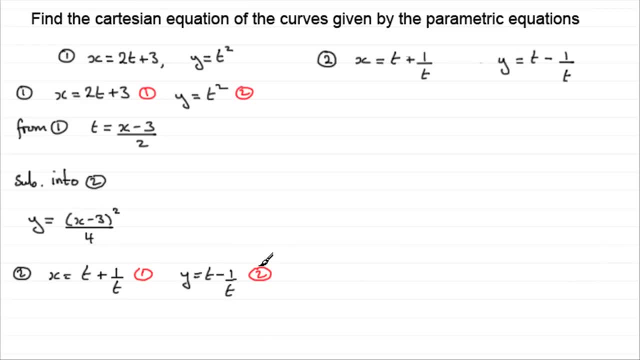 eliminate T between these. Well, because T occurs a couple of times in each one of these equations here it becomes quite awkward to eliminate if you try and make T the subject from this one or this one. So the way round this is to notice that we can eliminate. 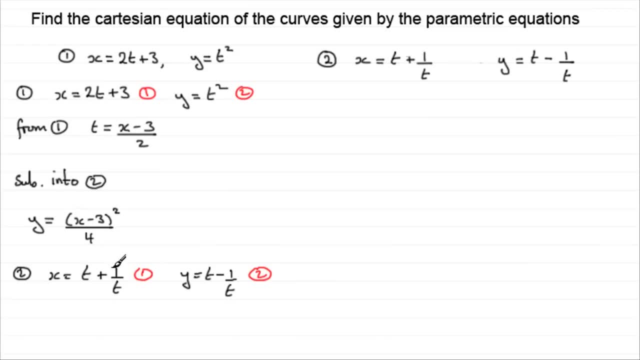 say this term here, the plus one over T term, with this term here, just by simply adding the two equations together. so if we do add them together, let's just say we do one plus two, what does that give us? Well, we'll have X plus Y. 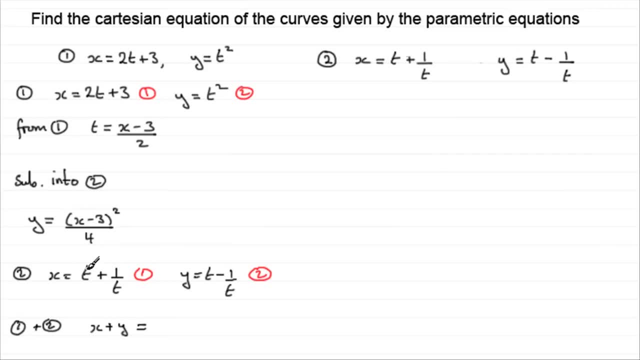 equals. and then we've got this T plus this T, so that's going to be two T and we're adding them because one over T added to minus one over T just cancels it out. So what we can do from this equation is now make T the subject. Well, we'll have to come down here. 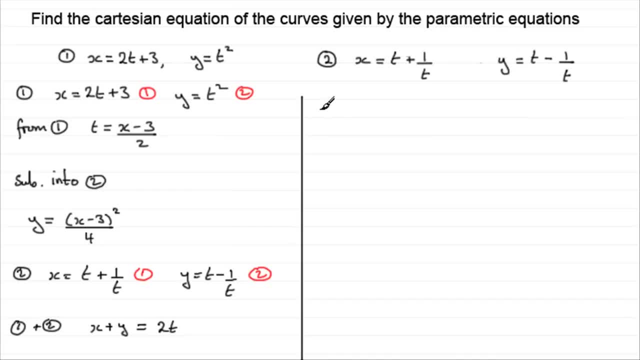 so if we make T the subject, by dividing both sides by two, we end up with T equaling X plus Y, all divided by two. Now I can substitute this either into this equation here or this equation here: one or two, It's up to you. I'll substitute it into. 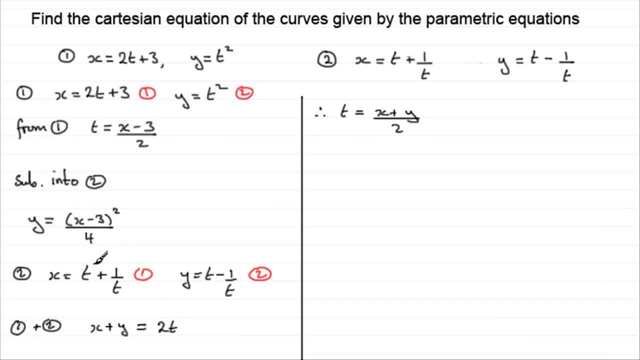 say equation 1 here, which is this one here? OK, and you might like to try substituting two and see how you get on. So let's say sub apostle одним into equation one. so we've got x equals t, t being the x plus y over two. 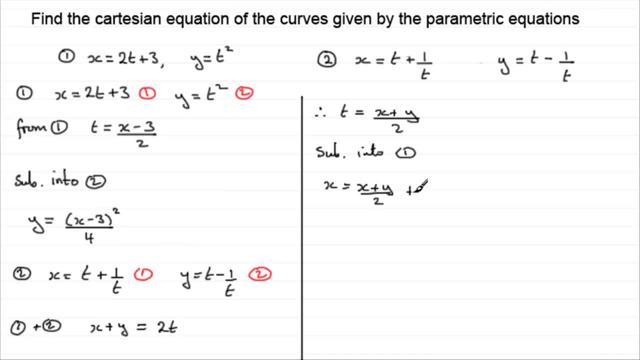 and then we're adding one over t. now, when we do one over t for this, it's going to be two over x plus y. we can invert it, so let's just write that in there. now we could leave it like this: we've got a cartesian equation, we've eliminated. 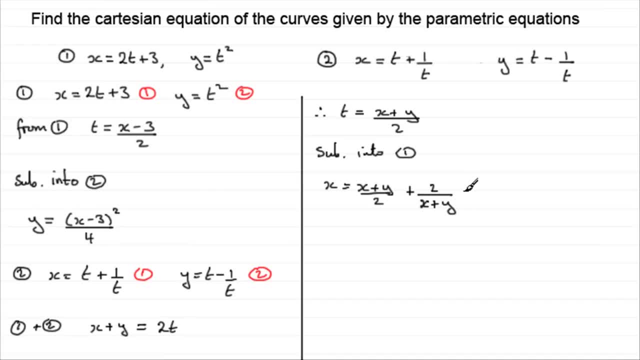 the parameter, but we might like to just carry on cleaning this up. we could multiply each of the three terms by two and x plus y, two bracket x plus y. so when we get to this one, we're going to have two x bracket, x plus y equals. and when we take this term and multiply it by two, 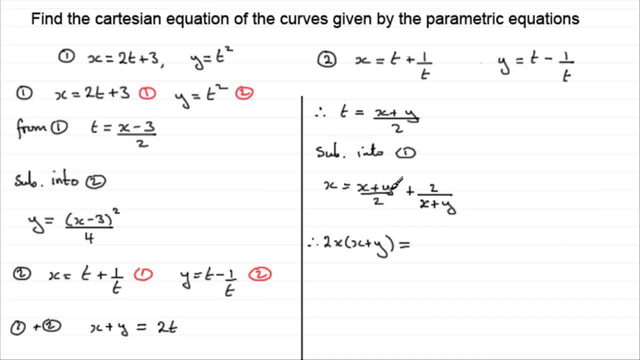 bracket x plus y, the two gets cancelled and we have x plus y all squared and for this term, the x plus y gets canceled and we end up with two times two, which is four, and i'd multiply this out. so we therefore have two x squared plus two x y. 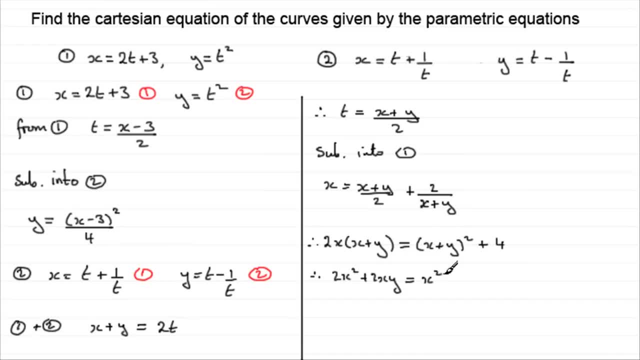 equals and if we square the bracket we're going to get x squared plus an x, y and another x, y, 2xy, and then plus the last term squared, y squared, and then the plus 4, and you'll notice now this is quite nice because the 2xy's are the same on both sides of the equal, so they get cancelled. 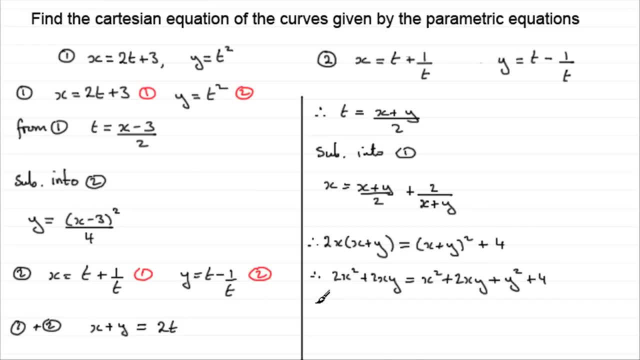 we can take x squared from both sides and we get x squared. we end up with equals y squared plus 4. we could subtract 4 from both sides and we end up with y squared equals x squared minus 4, and I'll leave it like that. 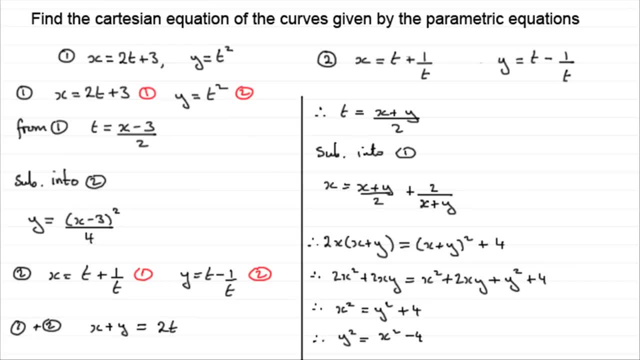 that looks quite nice. we have our Cartesian equation, okay, so I hope that's given you some idea where we have the very easy substitution here. but in this kind of set up you might have to modify the equations to eliminate one of the t terms. okay,